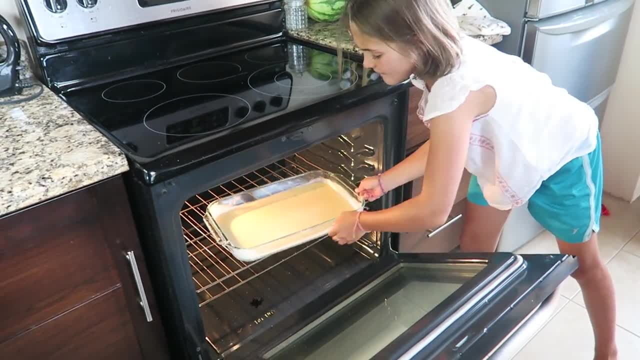 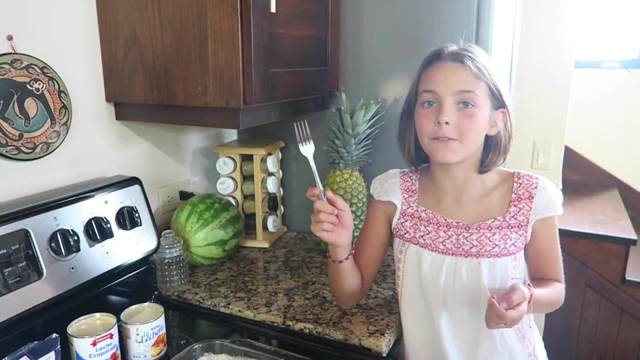 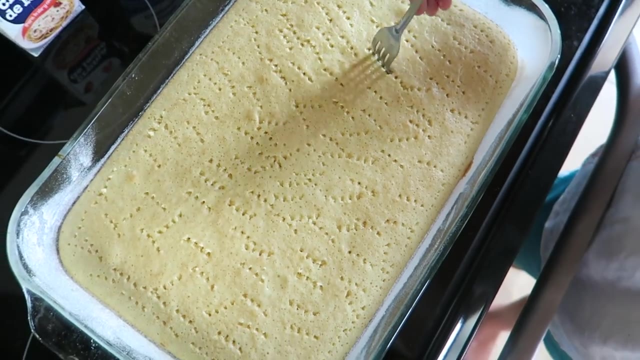 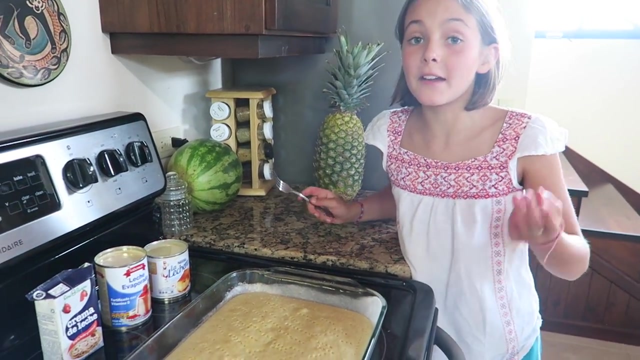 Let's get it to the oven- it goes. So I just got our cake out of the oven and now we're going to poke holes in the cake with a fork. See all of those pretty little holes. Alright, now we're going to put the milks in. 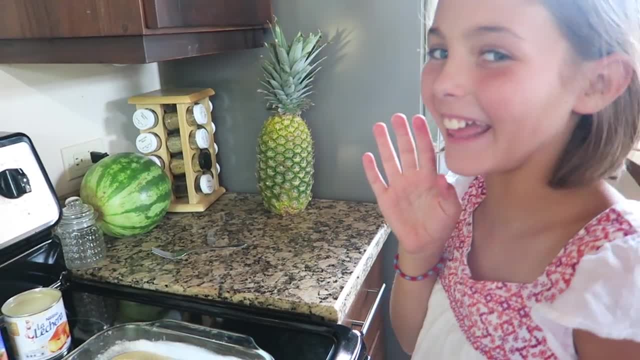 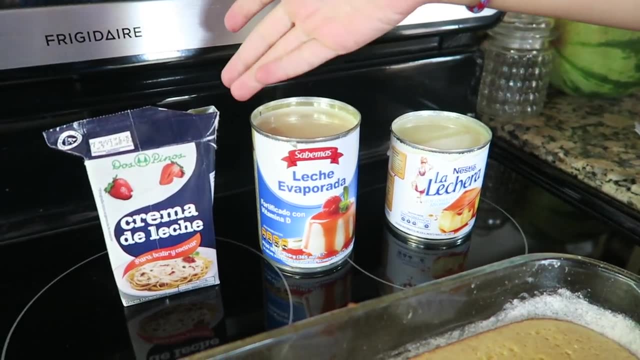 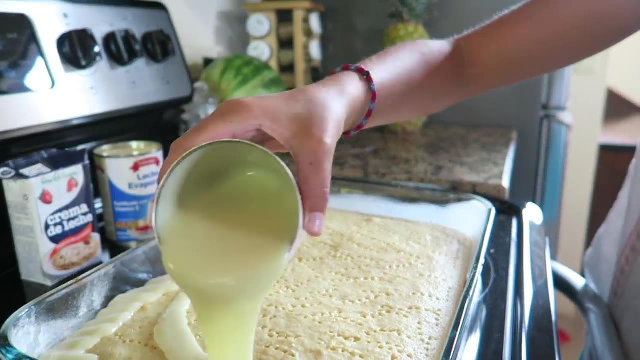 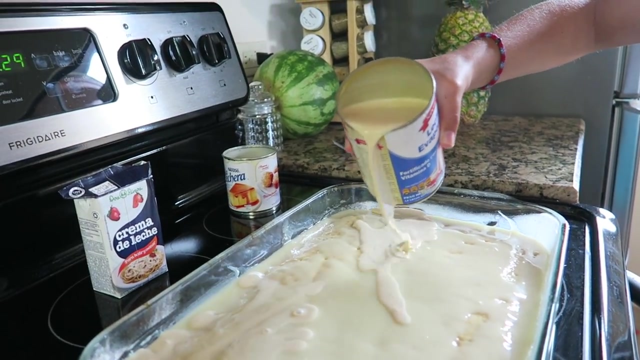 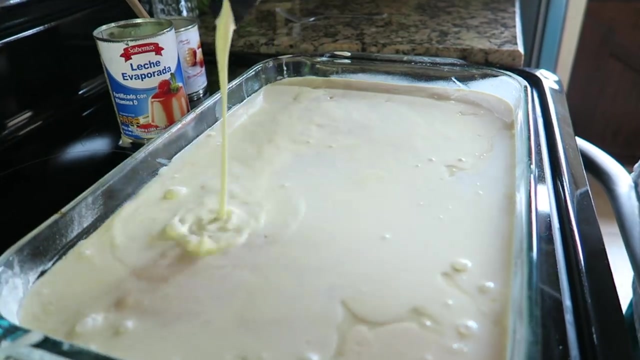 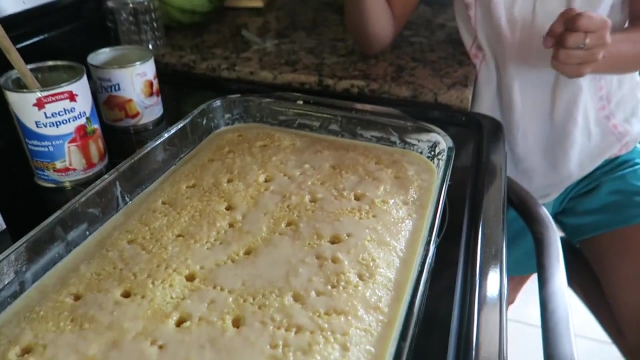 I have three different kinds of milk: Tres leches. This one is called sweetened condensed, This one is evaporated leche And this one is cremé de leche. Now it's tres leches, baby. Here we go see how the cake, totally like, sucked in all of the milks. 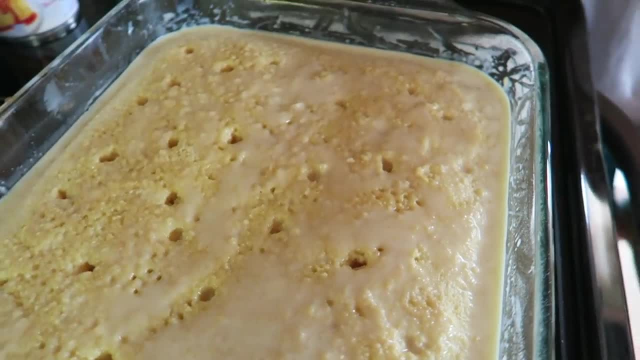 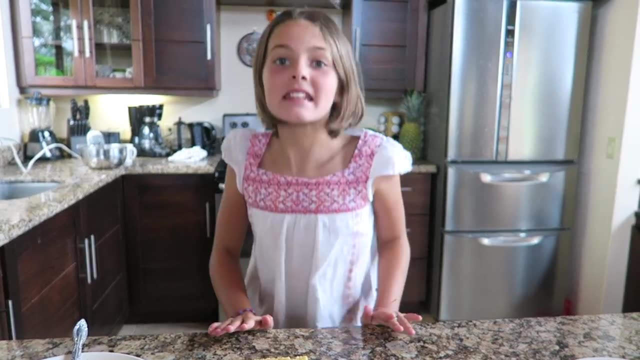 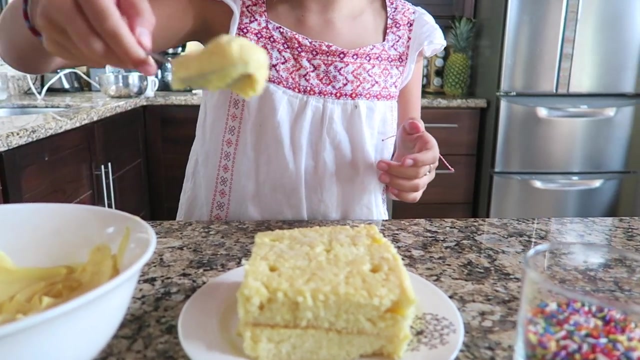 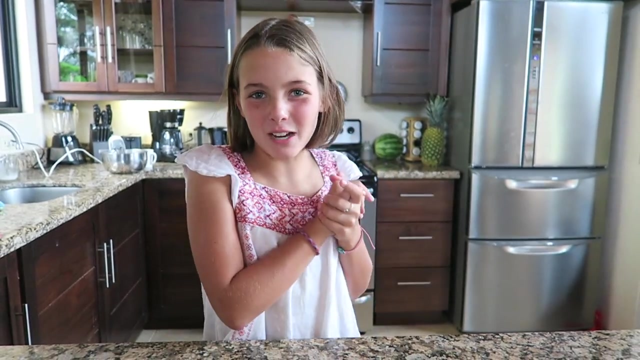 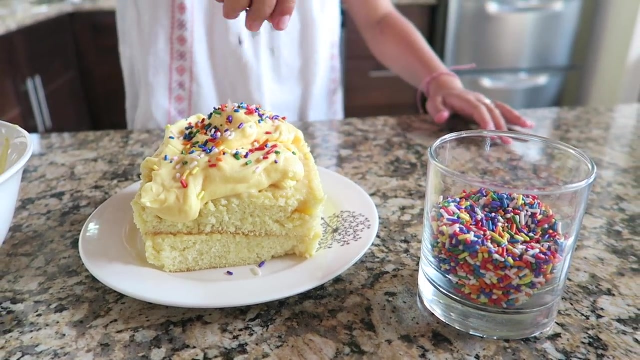 It acts like a sponge. that's so cool. oh, that looks so yummy. Alright, now let's move on to our toppings. Now time to decorate. So we have here some whipped cream. alrighty, Now time for the sprinkles. oh, this looks so good. oh my gosh. 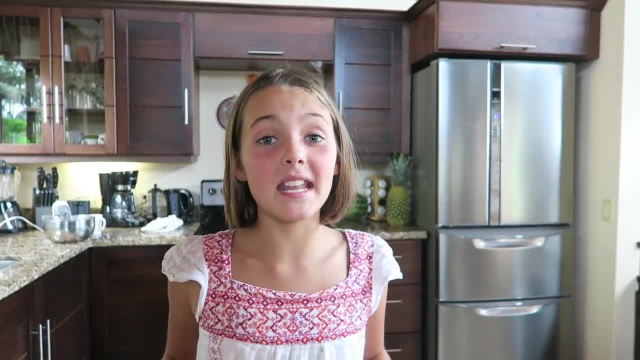 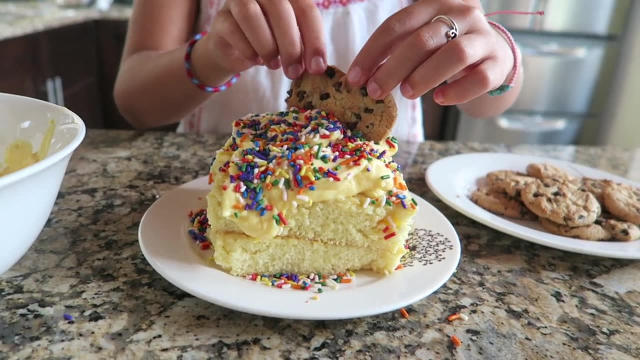 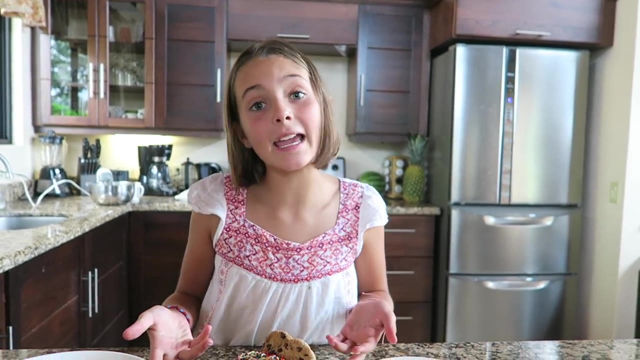 I told you I love sprinkles. Last but not least, what goes good with milk? of course, cookies. here we go, ta-da, our Tres Flechas cake is finished, but we can't have a cake without a party, so let's go have a. 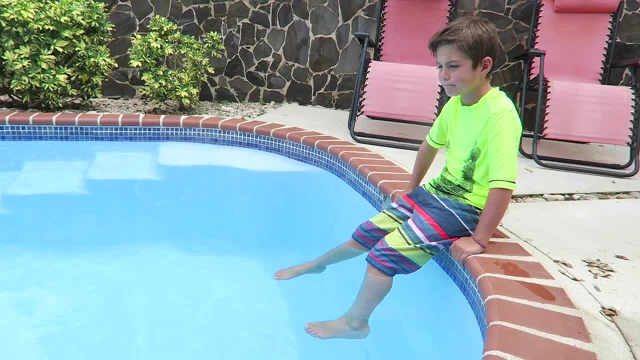 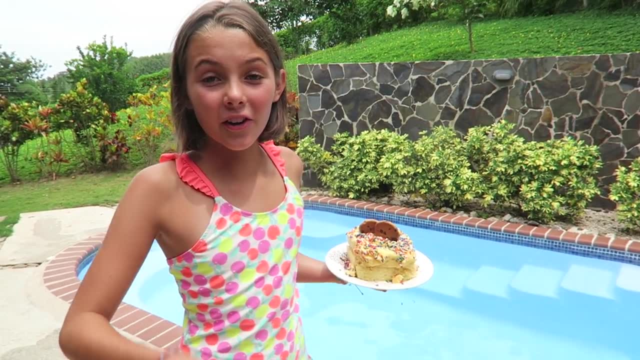 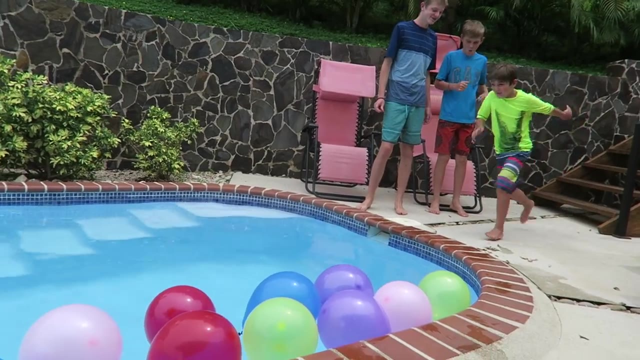 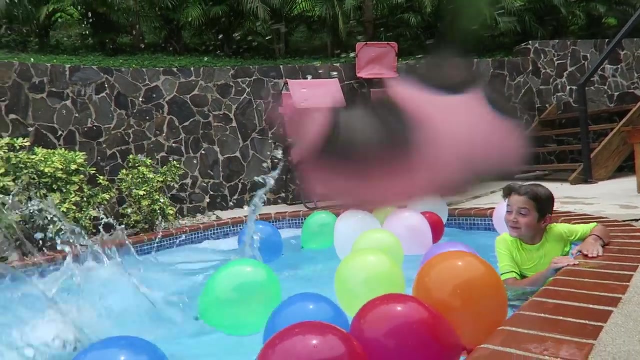 party. Hey, Axel, do you want to have a party with me? Yeah, sure, Ready. one, two, three, Oh my gosh. Oh, this is awesome Party time. Oh my gosh, oh my gosh, oh my gosh.